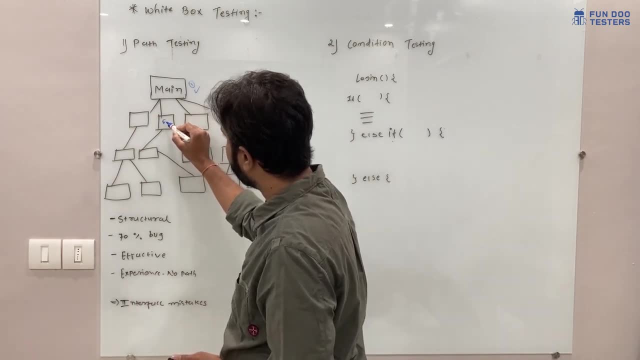 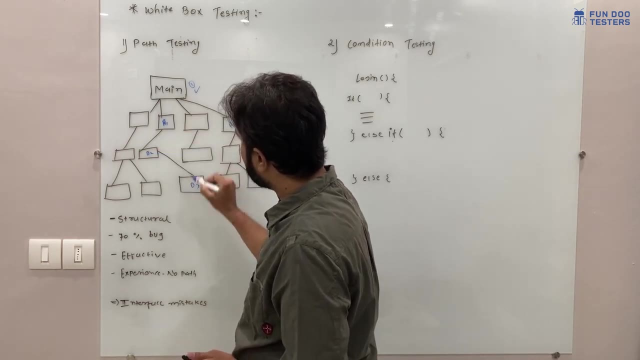 here. this will be a, for example. this is the f, this will be a a1, this will be a2, this will be a 3, like that we can make a path. this is on b1, this is b two. so this is going to from, this is from the f, so f a1, f, a 2. 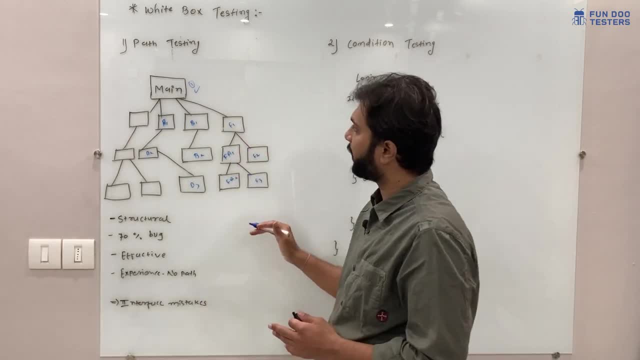 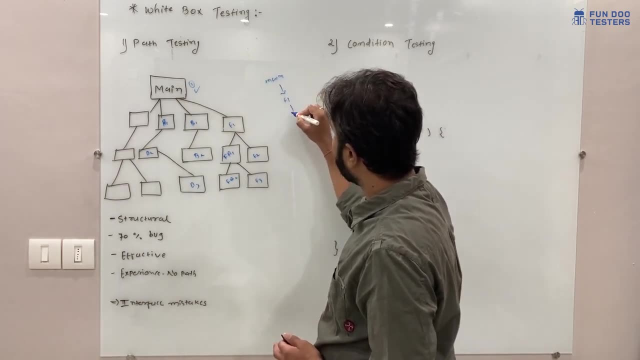 so like that they are going to. we can make multiple paths. so how we need to test. so first we are going for a main function, so this we are going to go: This will be the main function, then F1, and then F2 and then F3.. 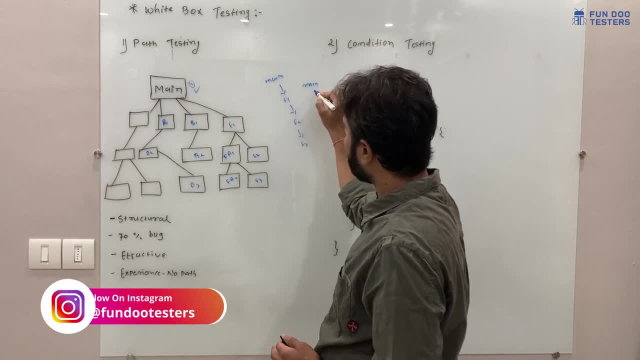 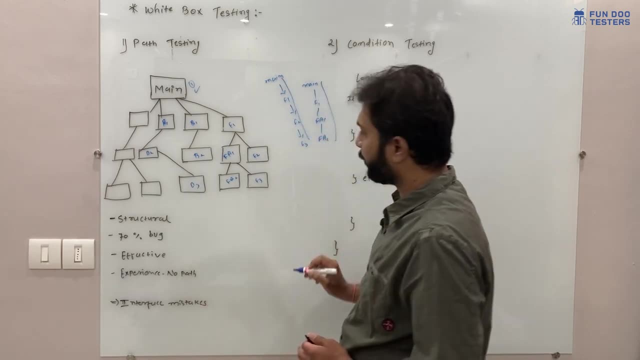 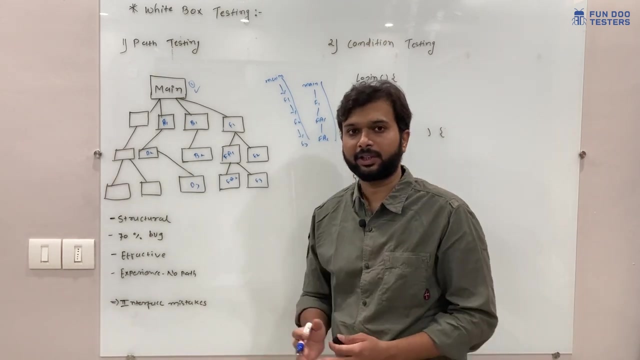 Other paths we can make as a main function, then F1, FA1 and FA2.. So this: we have two different paths, So we need to test these two paths. So the thing is, path testing is a structural type of testing. 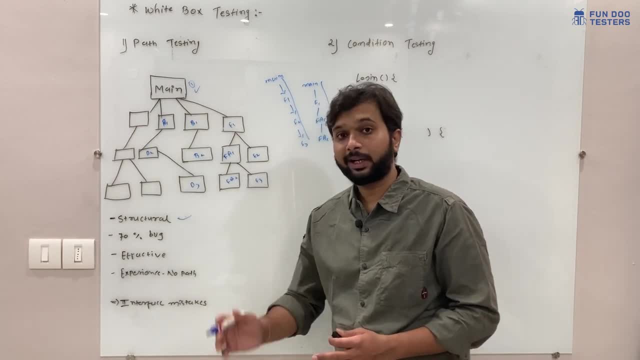 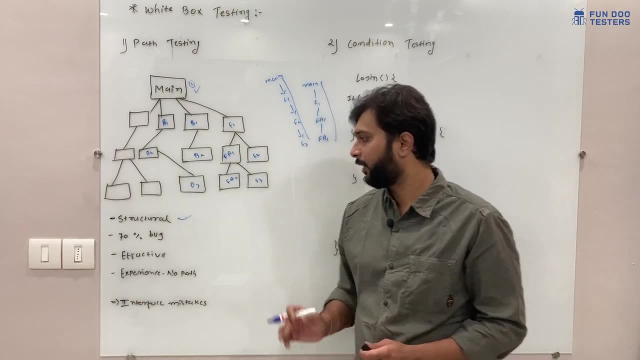 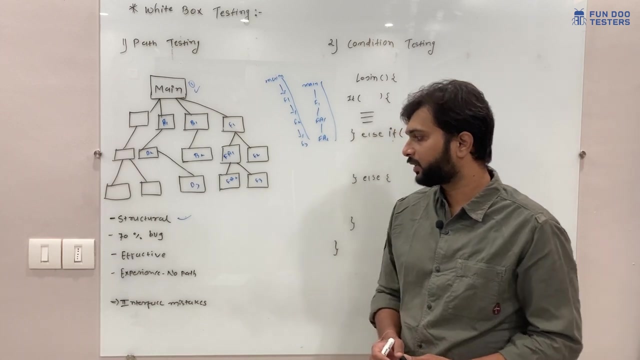 So in that case in this structural testing we can find out more than 70% or 60% defect. we can find out in the path testing itself And this testing is more effective as compared to the other white box testing. And in path testing, for example, developer is experienced. 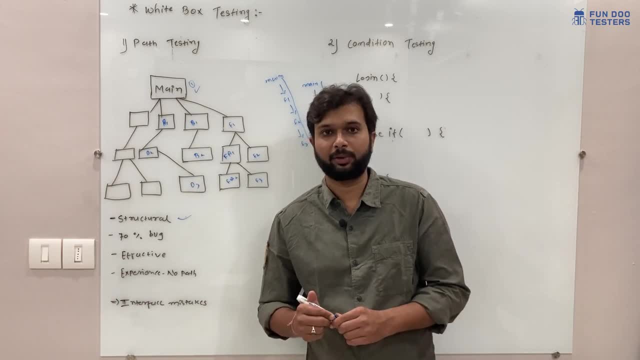 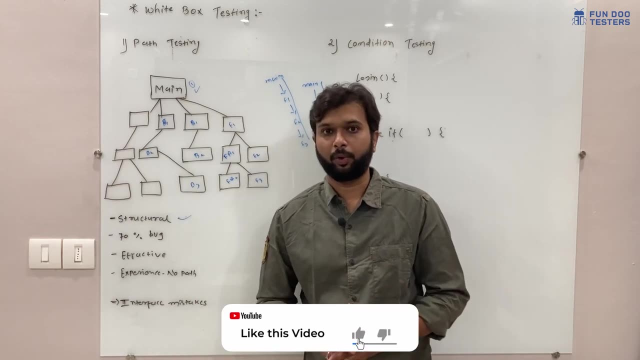 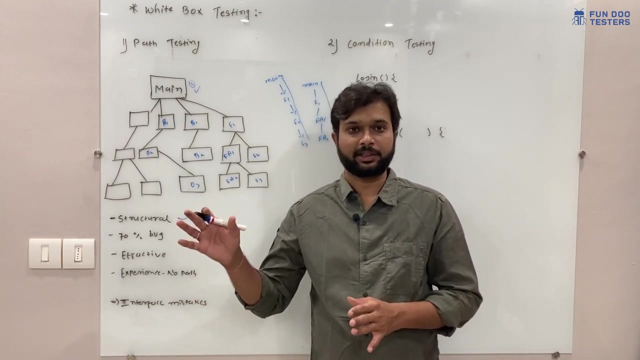 Generally what happens? some newbie developer, for example, truthier guy, has written the code. So what happens? architect level or senior manager level Will review their code. So if person is experienced, technical, very technically sound and architecture level person or manager level person, 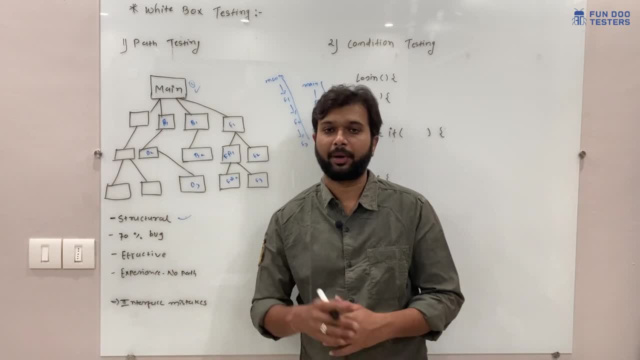 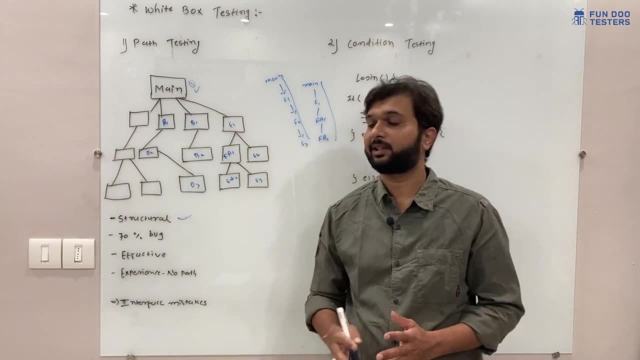 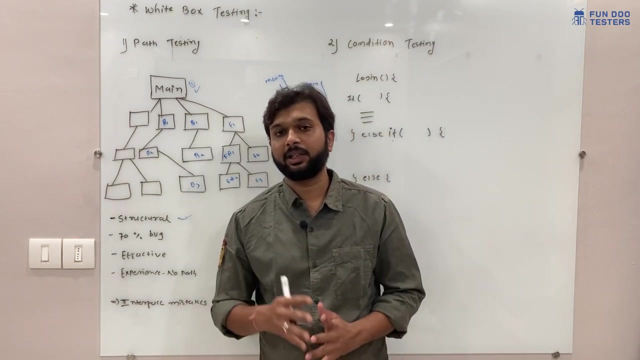 For that person, no need to draw the path. They can easily understand the path from where it is going. from where to where it is going. They can easily understand the path And there are few limitations In the path testing. they cannot face the error. 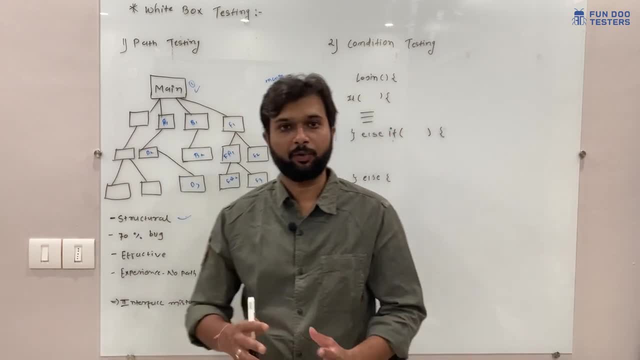 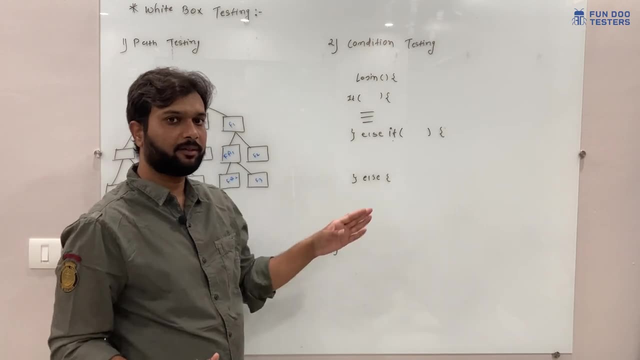 And there are few interface level mistakes. So this is all about the path testing. Now we are going to move on the conditional testing. Let's say I have created one login function. So what happened in the login function or any other function? 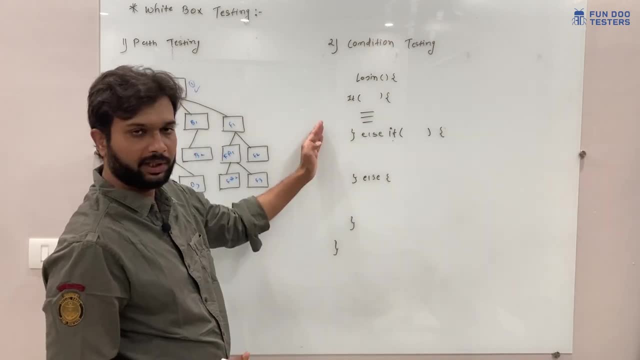 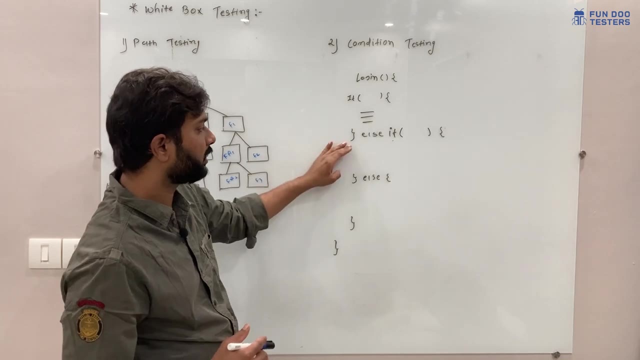 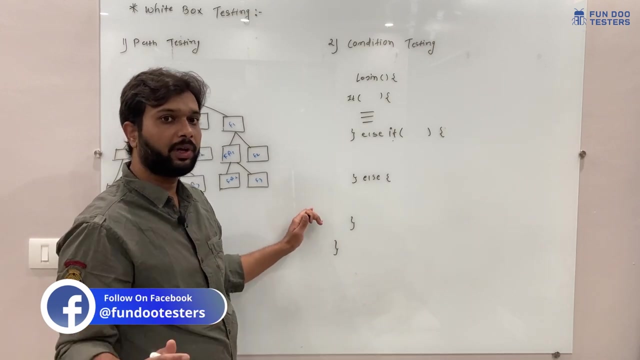 I developer has written few lines of code. So in the E there are multiple switch statement we have, or conditional statement we have. So for example, they have written if statement else, if statement, else statement. So in that case what happened? they have to go through the each and every scenario because for the end user,